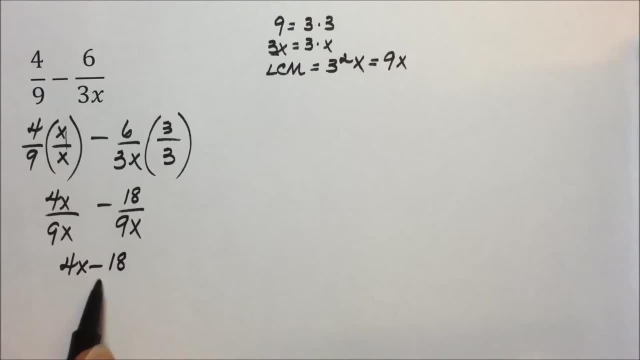 have common denominators, we can combine the numerators over that common denominator and we're done with the exception of always simplifying your rational expression. To know whether this is reduced, we'll factor first in the numerator. greatest common factor is 2, leaving 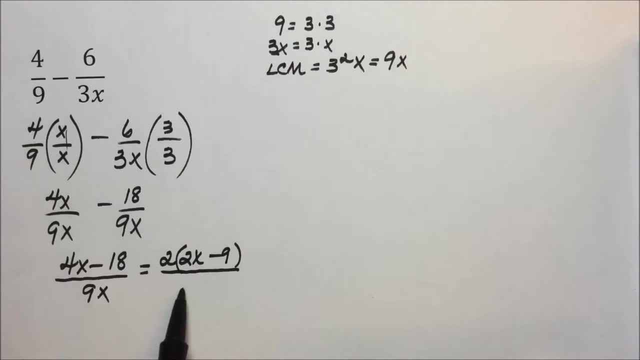 a 2x minus 9 over the common denominator of 9x. nothing to be done there. And looking numerator and denominator, there is no binomial. 2 and 9 don't have anything common. but it's clear now, because it's in a factored form, that it is simplified as far as it can go. 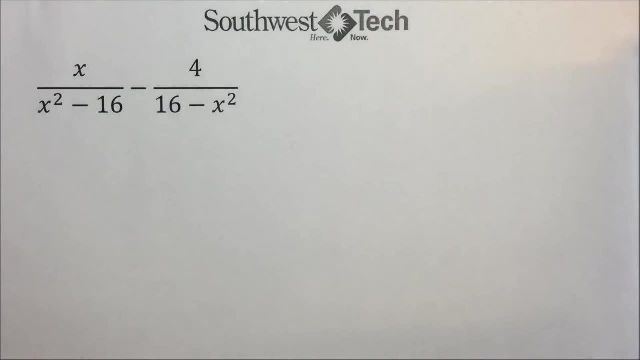 This next example is a subtraction of two rational numbers with unlike denominators, but they're still clear. If this 16 was only a negative 16, and if this x squared was only a negative a positive x squared, they'd be exactly alike. Well, if you remember from factoring, we had a technique. 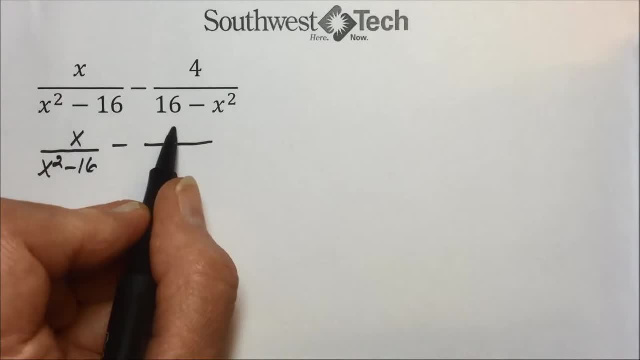 that changed the signs and that changing of the signs was factoring out a negative 1.. Factoring out a negative 1 changes the 16 into a negative 16,. factoring or dividing a negative 1 changes the minus x squared into a plus x squared. We now have same terms. 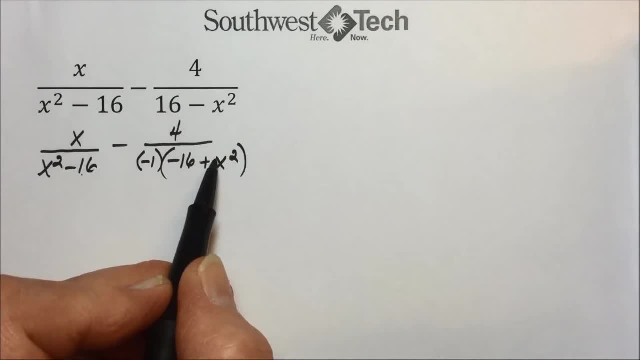 and just to verify that, do your distributive. we're back to what we had, Simplifying this. we have our original rational expression, nothing changed. but we have a positive divided by a negative is a negative. subtracting a negative turns into a plus, Minus and minus. 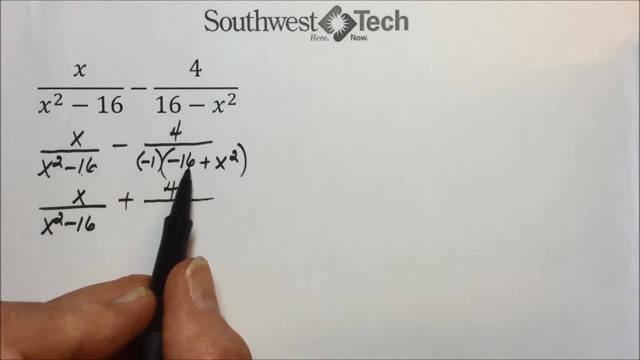 is plus 4 in the numerator. And while we're at it, let's rearrange. let's put our x squared first and the minus 16 second. So again, this subtraction, with this negative canceled out giving us a positive. We now 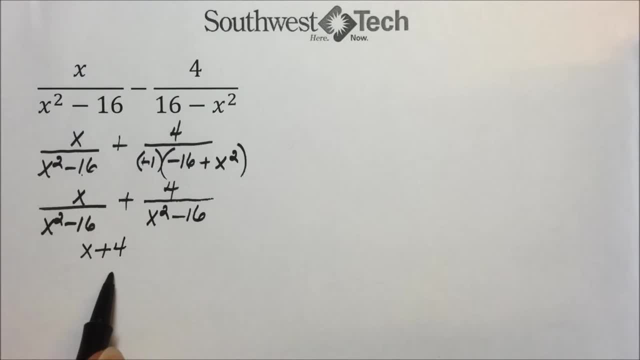 have common denominators. we can combine the numerators And always on guard for simplifying or reducing the fraction, The numerator, there's nothing to be done. but in the denominator we have a difference of squares Which factors into an x minus 4 times an x plus 4.. 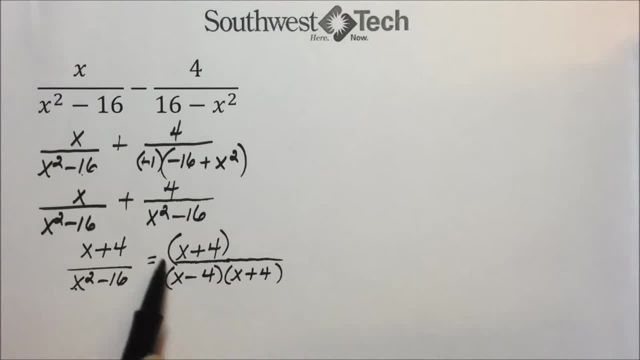 And now, looking in the numerator and the denominator, we do have a common binomial factor of x plus 4.. When you have the same thing over the same thing as a factor, it cancels out, leaving a 1.. Our final answer then is 1 over x minus 4.. 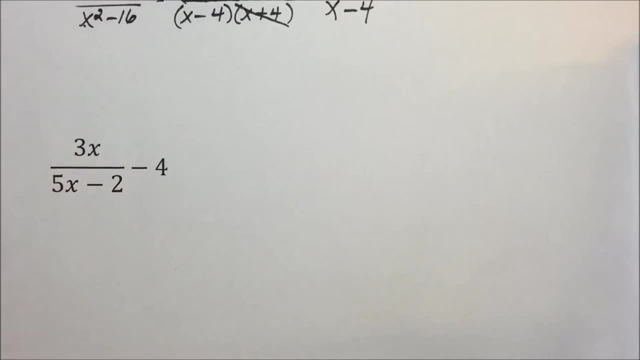 In this next example we have a rational expression minus another rational expression minus another rational expression, where the second fraction has a denominator understood to be 1.. So our least common multiple of the denominators is simply 5x minus 2.. 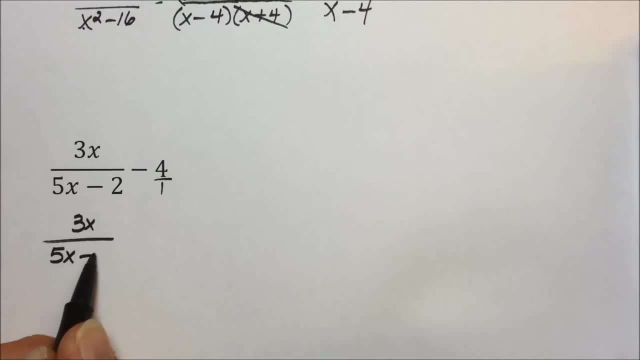 The first fraction needs- or rational expression needs- nothing done to it. The second, however, needs a factor of 5x minus 2. So that we can get the common denominator. And if the denominator gets multiplied by that quantity, so does the numerator. 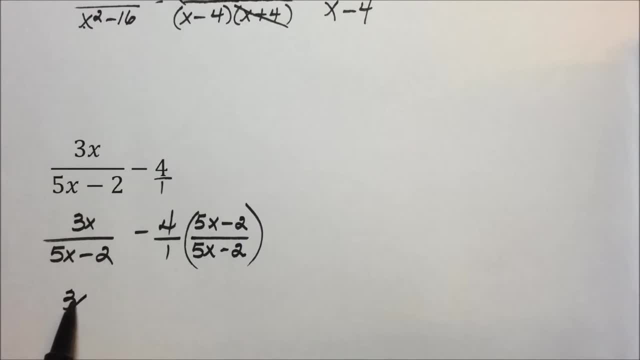 So essentially multiplying by 1.. We can then do a simplification. This subtraction can be thought of as plus a negative and distribute, so we will end up with a negative 4 times 5 is a negative 20x, A negative 4 times negative. 2 is a positive 10x. 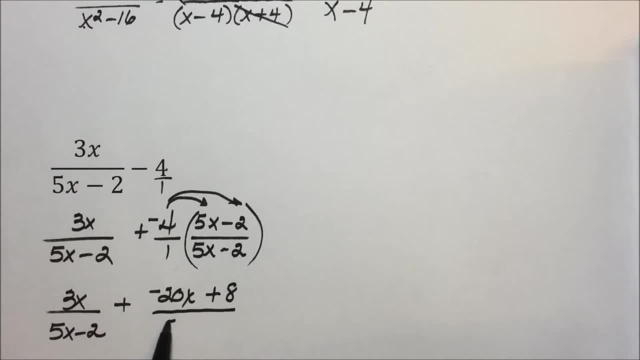 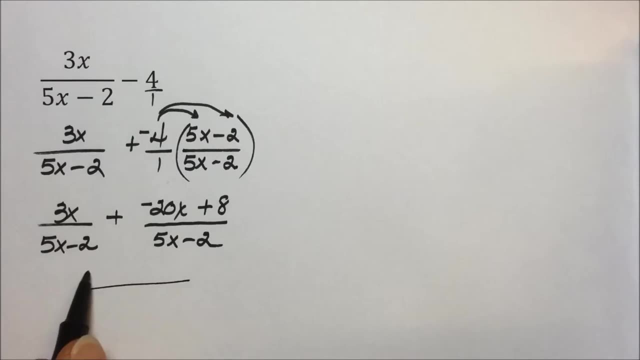 of 8 over the common denominator. We have our common denominators, so we will combine the numerators 3x plus the negative 20x plus 8, all over the common denominator of 5x minus. 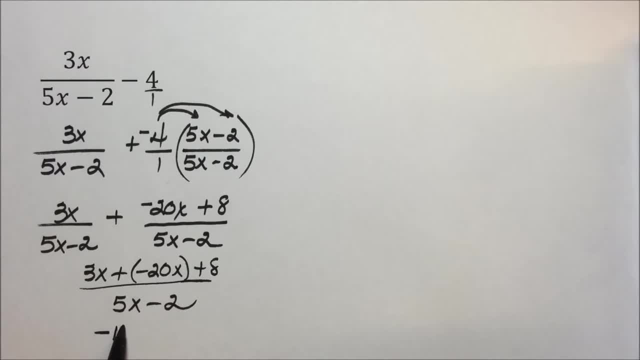 2. Simplifying: we have a negative 17 when we combine our 3x and minus 20 plus the 8 over 5x minus 2. Factoring-wise to see if we can simplify: 17 and 8 have nothing common. 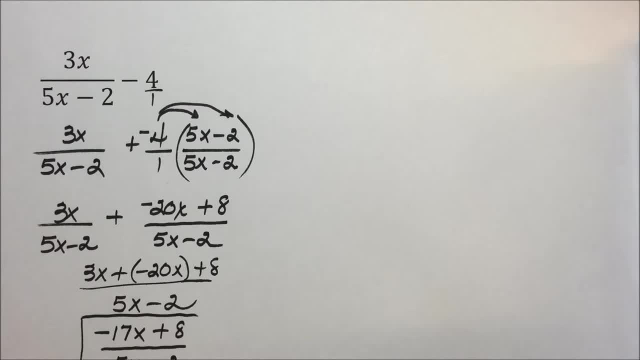 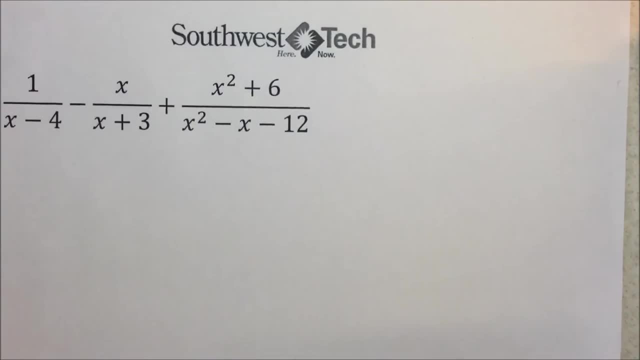 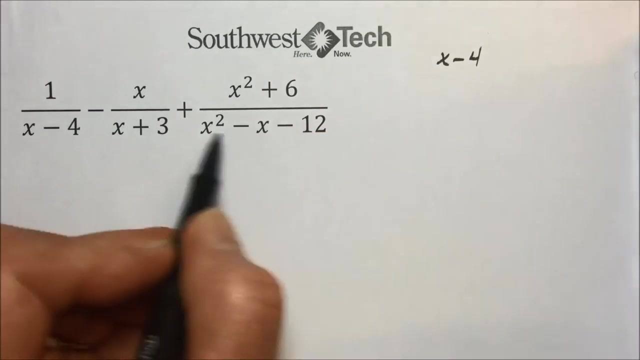 neither do the 5 and the 2, so this is our simplified rational expression for that operation. In this next example we're adding and subtracting rational expressions. We're looking for our least common multiple. The first fraction: it's clear, it's an x minus 4.. The second fraction's denominator: 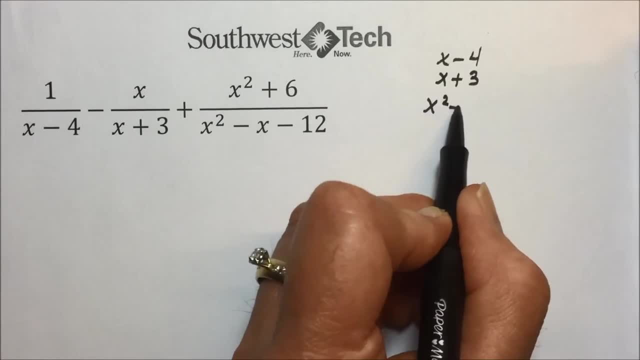 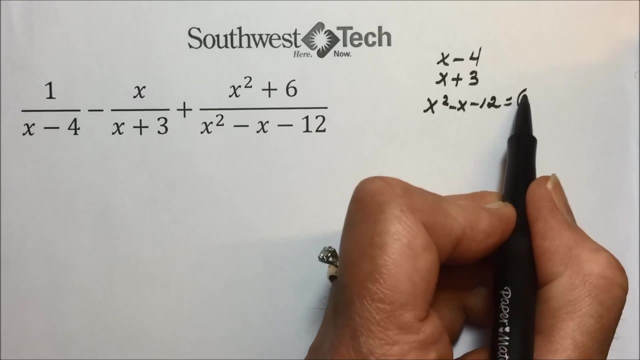 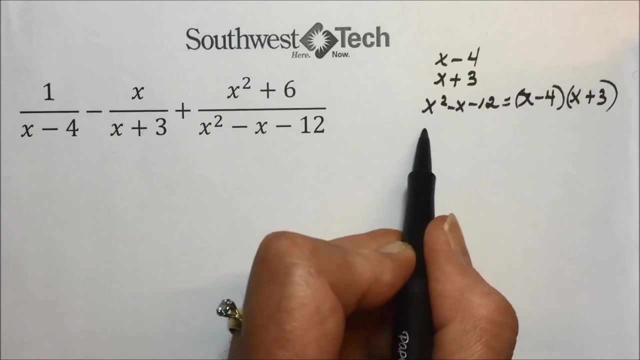 is an x plus 3.. And if we factor x squared minus x minus 12, it factors into an x minus 4 times x plus 3.. Our least common multiple has to have these two factors. which good note. Subtitles by the Amaraorg community. 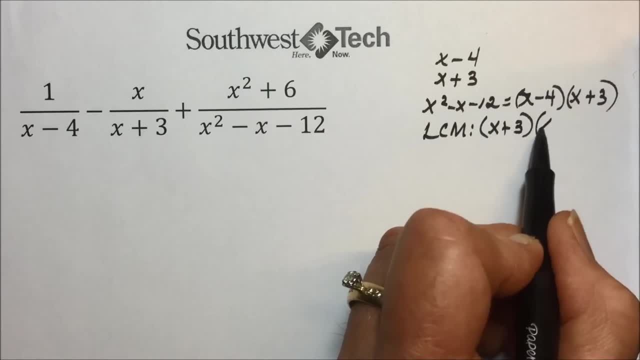 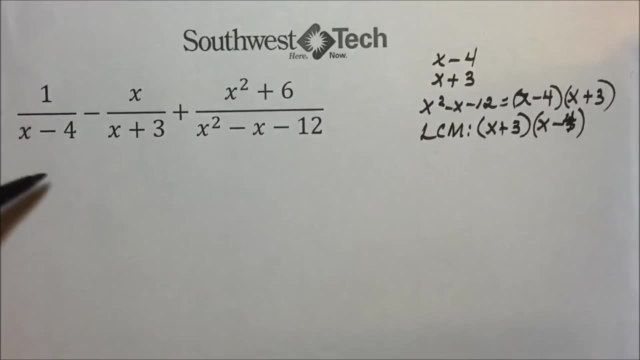 news is: whoops, I'm having difficulties. there apparently are that should be a 4, are the factors of these two rational expressions with only the binomial. So before we add, we need to change each one of these and subtract, we need to change each one of these rational. 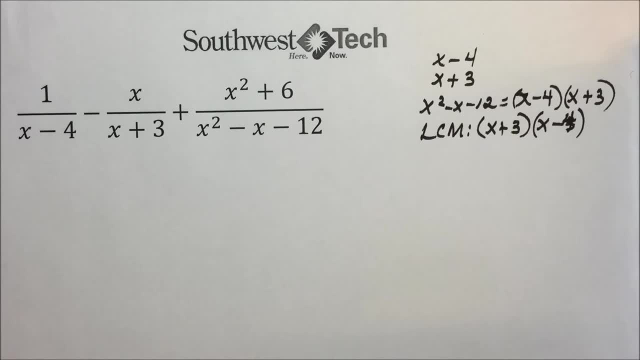 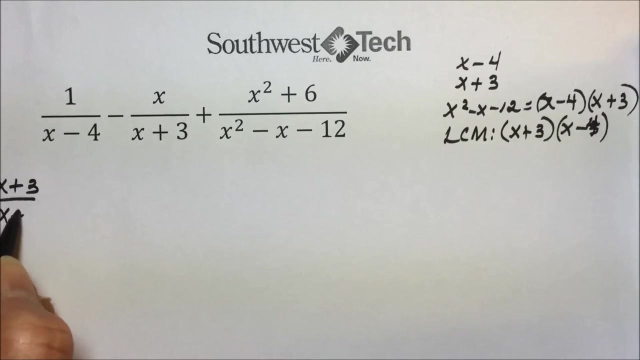 expressions so that they have that least common multiple. So our first fraction has the x minus 4, but it needs the x plus 3.. So we will multiply the numerator by x plus 3 and the denominator by x plus 3.. The second fraction needs the x minus 4 because it always has. 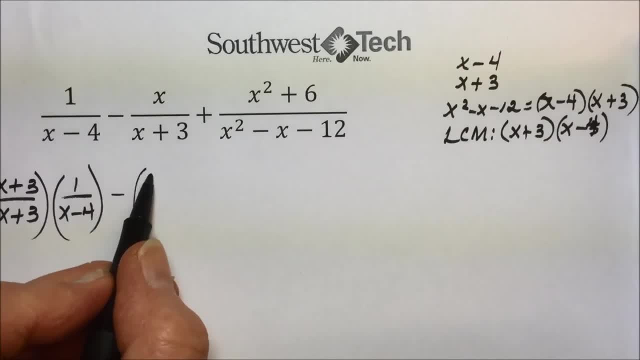 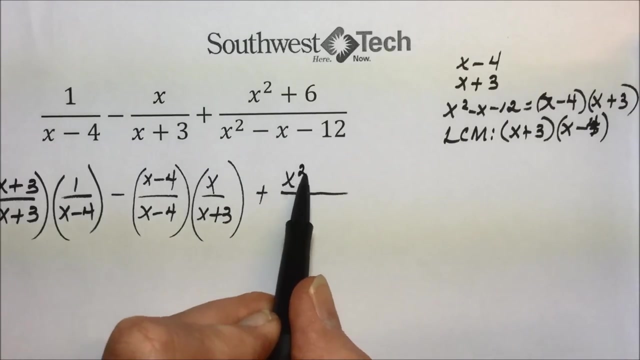 the x plus 3.. So we will multiply the numerator by x minus 4 and the denominator by x minus 4.. And the third fraction: here nothing needs to be done other than maybe replace. So we can see the factors of that denominator are in fact x minus 4 times x plus 3, so this: 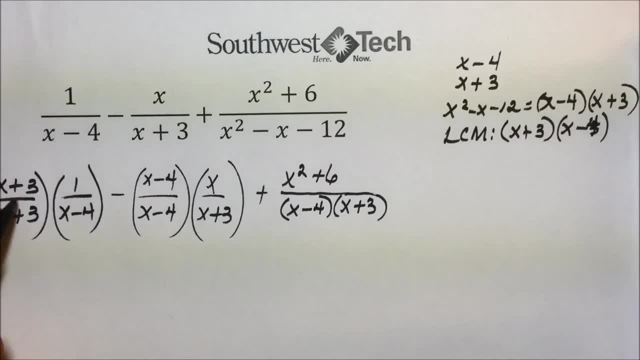 3. Each one of the first two fractions was multiplied by a very special one. that brings us up to a common denominator and simplifying that. we have an x plus 3 times 1 is x plus 3 over x plus 3 times x minus 4 minus. we have a distributive property here: x times. 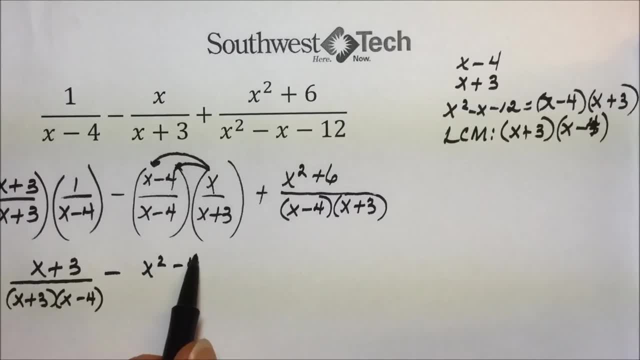 x is x squared x times minus 4 is minus 4 over the common denominator of and order isn't important. if you want to see that they're all uniform, we could put our x plus 3 first, followed by our x minus 4 plus. we did nothing with our last rational expression other than